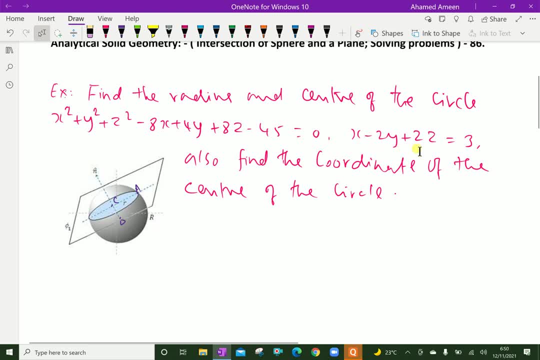 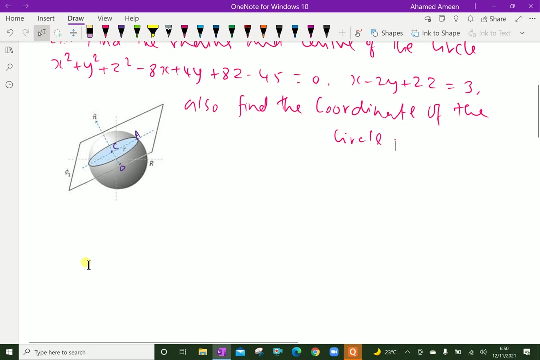 and the plan x minus 2y plus 2z, equal to 3.. Also, find the center of the circle Here. look at this figure: A sphere is intersected by a plan and it forms a circle in a common space. Now we write: given sphere is x squared plus y squared plus z squared minus. 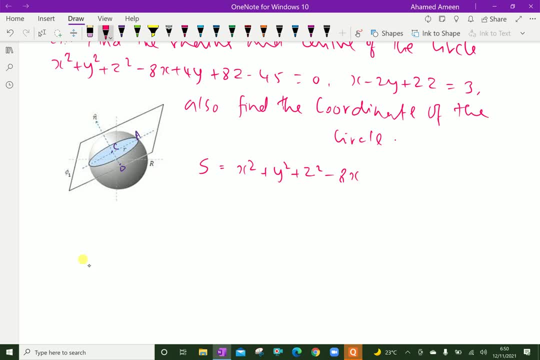 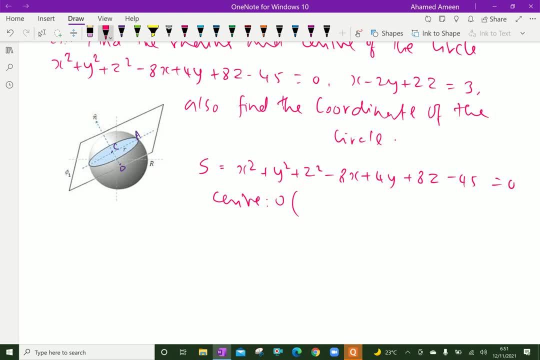 O is here, that is minus g. had to do minus f and h, that is 4 and minus 2, that is 4 by 2 is minus 4 by 2 is minus 2,. 8 by minus 2 is minus 4.. This is a center. 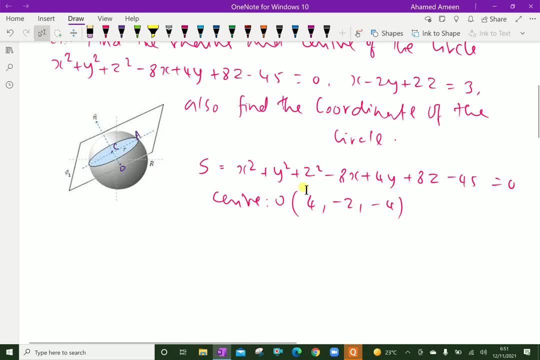 Now, and radius, radius of the sphere. radius of the sphere is square, root of this is. radius of the square is the 라� of the double square, which is Bagler cosine, and radius of the square is, you have to find that, this square, here, four square. 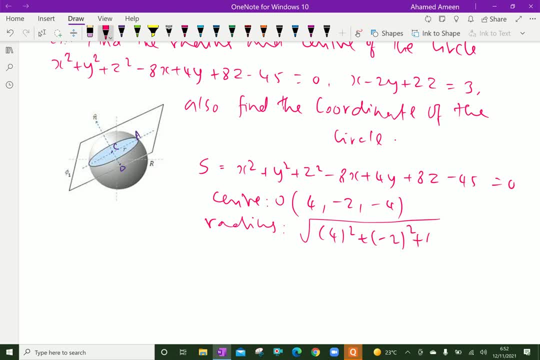 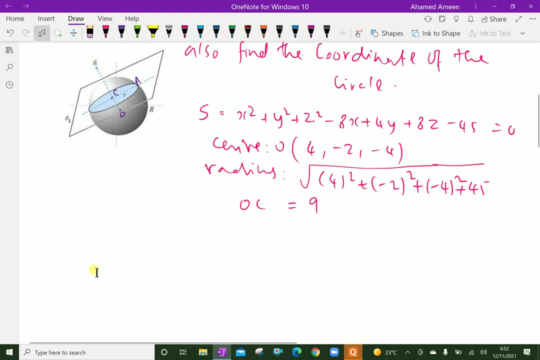 Now, plus minus 2 square, plus minus 4 square minus c, c is 45, minus 45. that is plus 45 here, which by calculation gives 9.. Here we found OC. Now we have to find the radius of the. 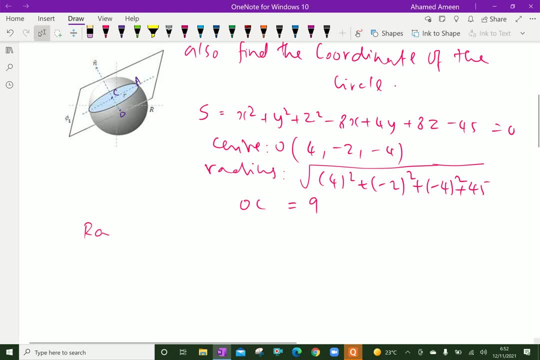 circle that is AC. radius of the circle that is AC. radius of the circle that is AC is the square root of. by Pythagoras was OA square minus OC square. Here, OA square minus OC square equal to c AC, which gives square root of 9 square minus 1 square, which gives 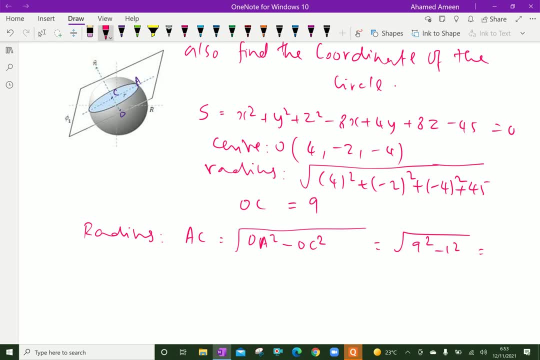 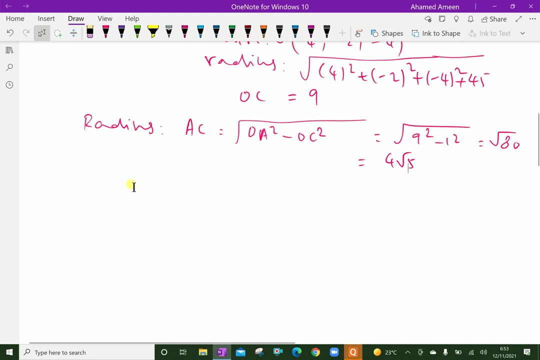 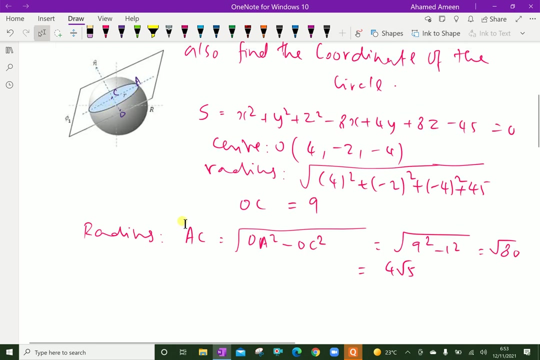 square root of 8. By simplification it gives 4 root, 5. Further coordinate of the center will find coordinate of the center you have to find. For that here OC is. OC is perpendicular to the plan. 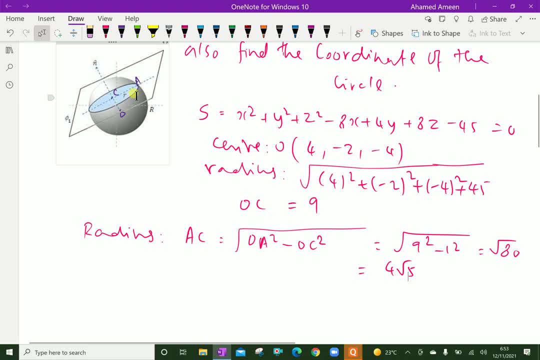 And we can say the direction plan of given plan, that is x minus 2,, y plus 2, z, equal to 3.. So the direction ratios of the line OC, OC are the same, those of the normal to. 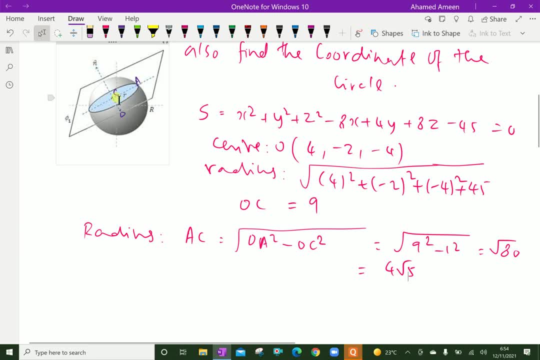 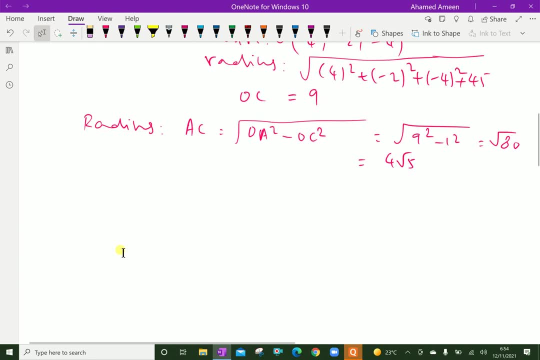 the plan. Here direction ratio of the OC is equal to direction ratios of the plan normal to the plan. That is therefore direction ratios of the plan. So the direction ratios of the of the given plan is 1, minus 2, and 2.. Therefore, and 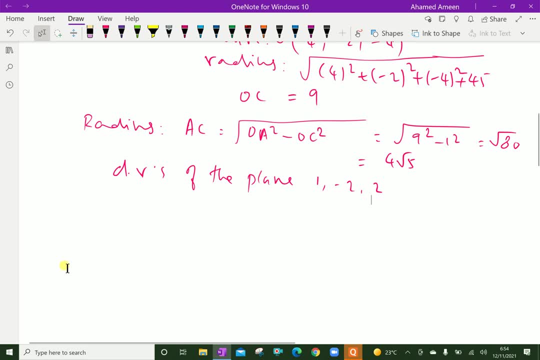 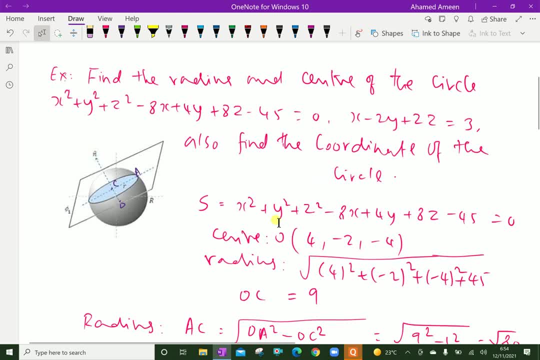 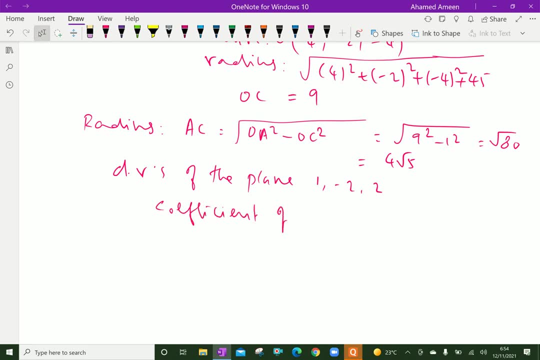 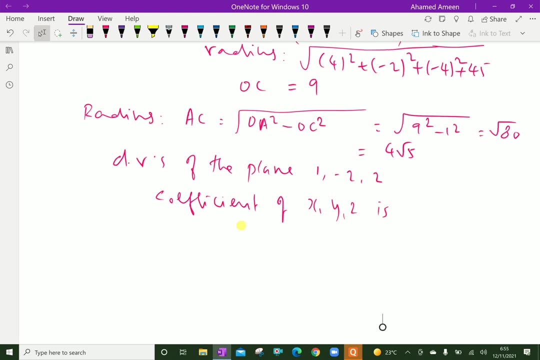 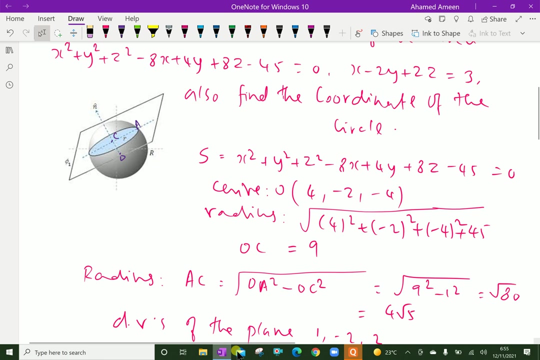 to is equal to: equal to 1 minus 1, and 2.. And the coefficient, the coefficient of x y z, s, x y z is 1, minus 2, and 2.. 1, 1,. 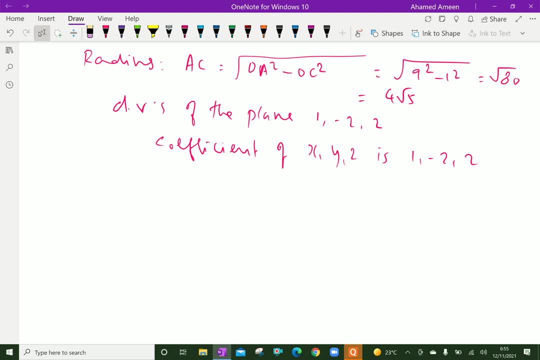 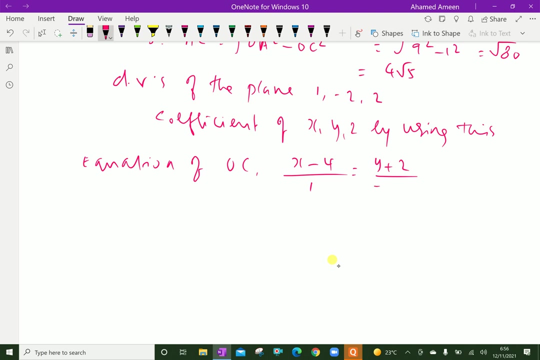 and 2. therefore, therefore, equation of OC, equation of or she can write X minus question. tough one question of XYZ is given and you can find by using: we can find equation of OC. this: we can find equation of OC that is: X minus 4 over direction ratio is 1 Y plus 2 over minus 2. 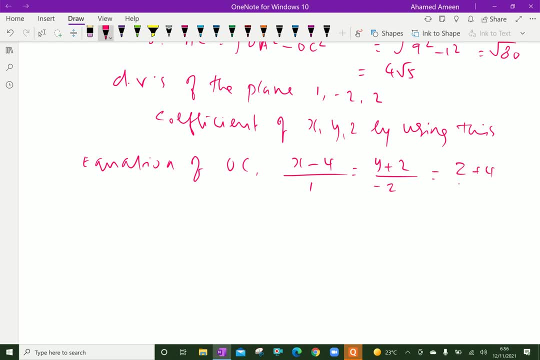 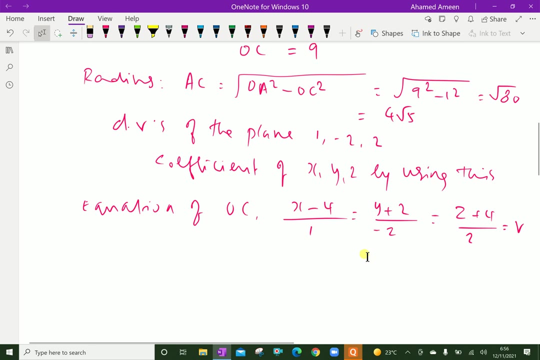 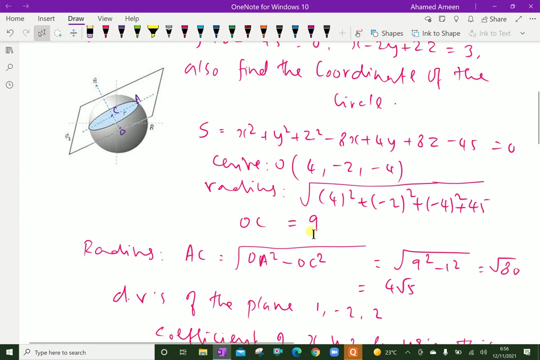 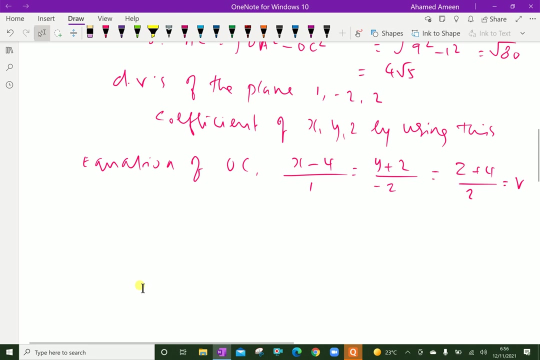 and Z plus 4 over to equal, say it is R. here these are coefficient direction ratios and this 4 to unfold this center. we are using this. by using these two coordinates we are finding the equation of the line OC. now from this we can find R, that is X comma, Y comma, Z. 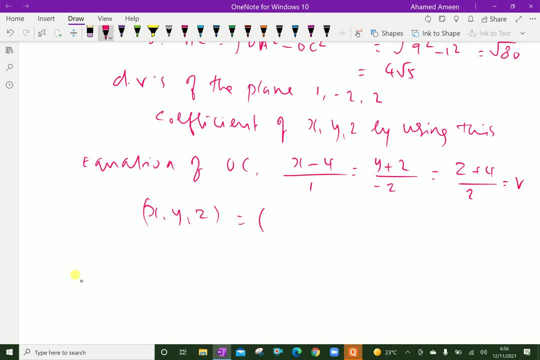 gives 1 R plus 4 minus 2, R minus 2 and 2 R minus 4. this is a, this is a coefficient of X Y Z. now, here these points lie on the plan. this point is on the given plan, given plane: X minus 2y plus plus 2, is it? let us? 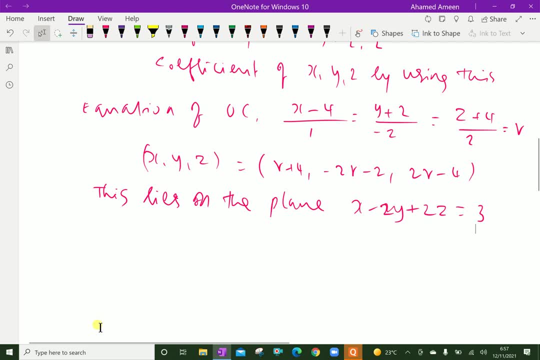 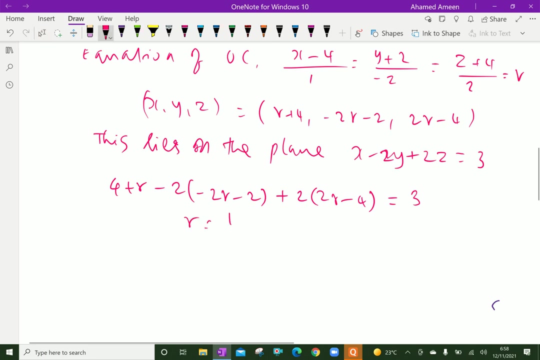 substitute this point, that is here 4 plus R minus 2, into Y value is minus 2 minus 2r, minus 2 plus 2z values, 2r minus 4, which is equal 3.. We are substituting this point in this plan So by using simplification and we will get r equal 1 over 3.. This 1 over. 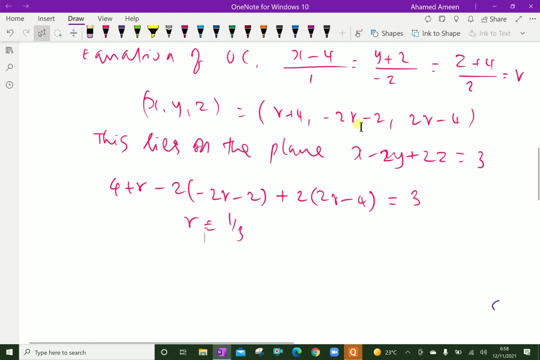 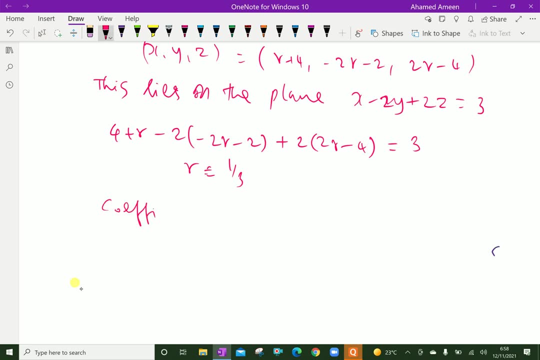 3. we have to substitute these points. that is center. we have Therefore coefficient of center of the circle, that is, we are substituting here this r in the center, like this: r is 1 over 3 plus 4 minus 2 into 1 over 3 minus 2 and 2 into 1 over 3 minus 4.. So by 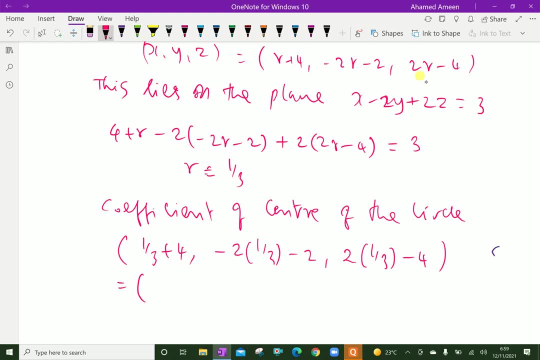 simplification, we get 13 over 3 and minus 2 over 3 plus 4.. So we get 13 over 3 minus 2 and 1 minus 8 over 3 here. that is 2 into 3, is 6 minus 6 minus 2, is minus 8 over 3.. 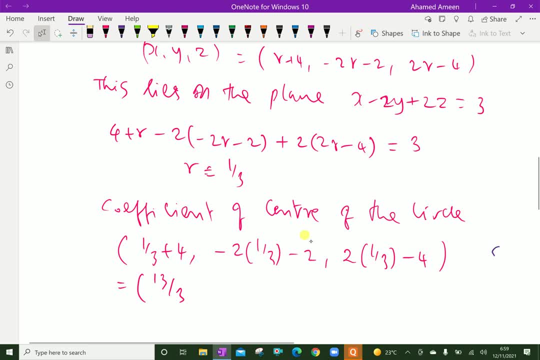 And here 30 is 2 into here 12. that is minus 12, that is minus 10 over 3.. This is a 3 over 3.. 14 over 3.. 15 over 3.. 16 over 3.. 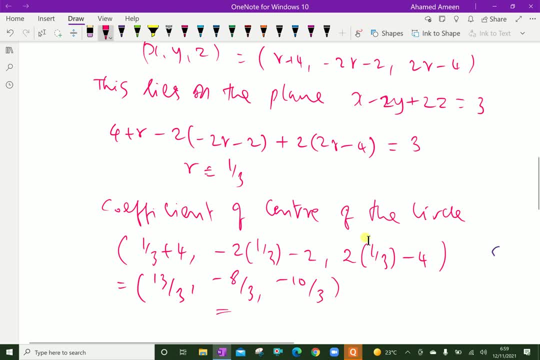 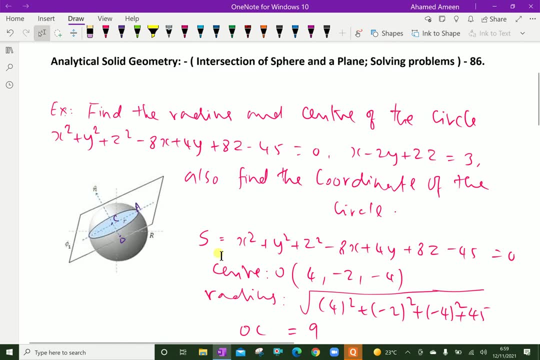 8 over 3.. 16 over 3.. 17 over 3.. coefficient of this coordinate of the center of the circle formed by intersection of a plan and this sphere. we have done. please subscribe our YouTube channel.